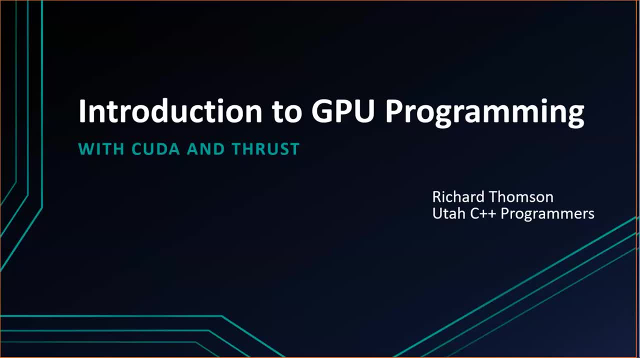 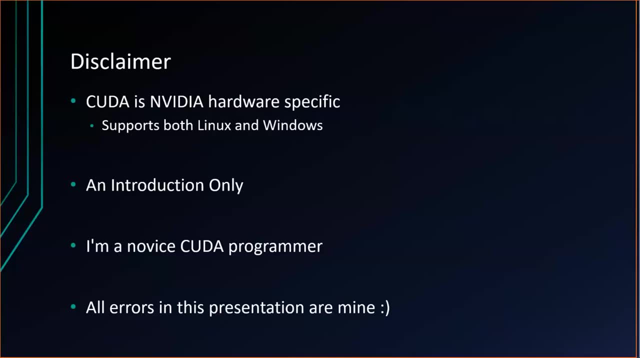 So CUDA is specific to NVIDIA hardware. I'm not aware of any vendor of other GPUs that provides a CUDA implementation. I've heard of CUDA translator layers that people sell, but I'm not familiar with those, so we're not going to say anything more about it. 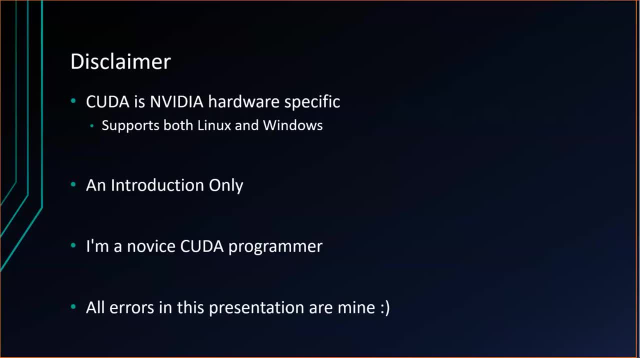 CUDA is supported by NVIDIA on Thrust, but it's not supported by NVIDIA on Thrust. So CUDA is supported by NVIDIA on Thrust, but it's not supported by NVIDIA on Thrust. This talk is an introduction only. CUDA is a very broad and deep topic and I'm only a novice CUDA programmer. I am by no means a CUDA expert. 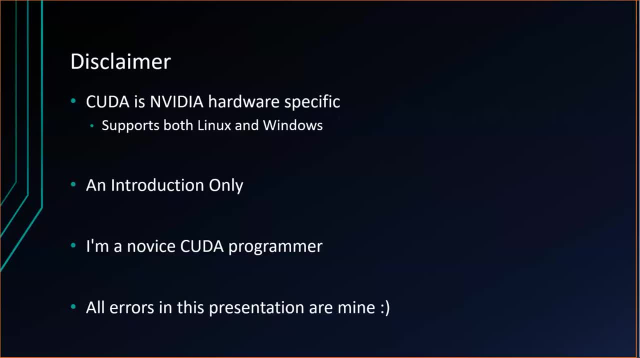 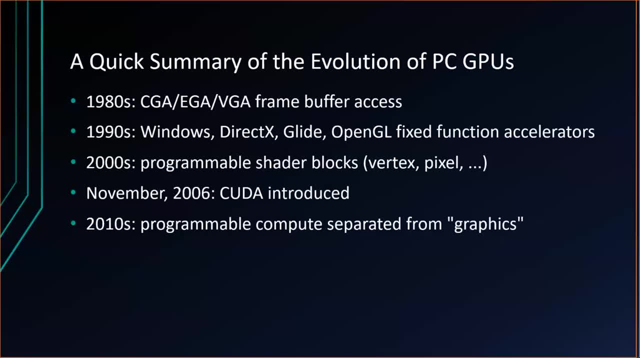 This talk is an introduction. only. CUDA is supported by NVIDIA on Thrust, but it's my fault and nobody else's. However, it's still trying to do general purpose computation by fitting this square peg of general purpose computation into the round hole of these shader blocks provided by graphics pipelines. 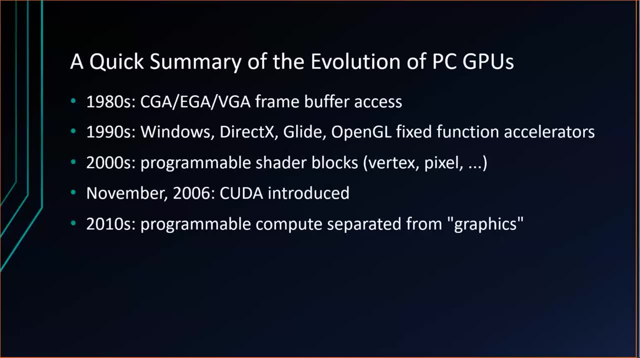 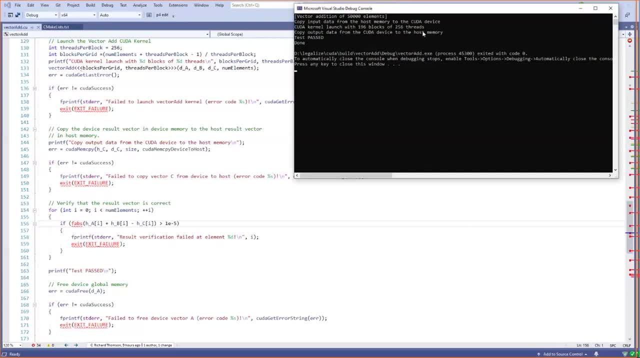 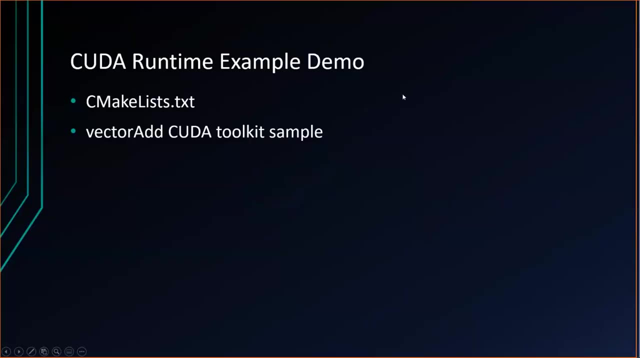 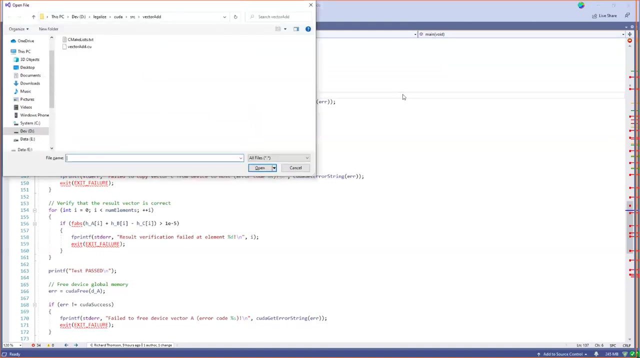 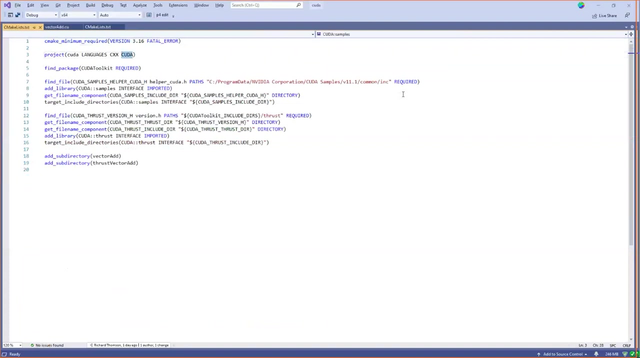 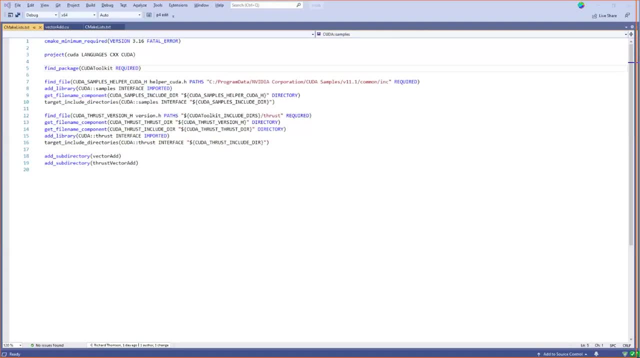 And excuse me, It's not required, but you can specify CUDA for your project as one of the languages that you're using. I do find package to locate the CUDA runtime library that I need to link against and the CUDA runtime headers. This stuff here I just added as a way to conveniently use the little helper file header. 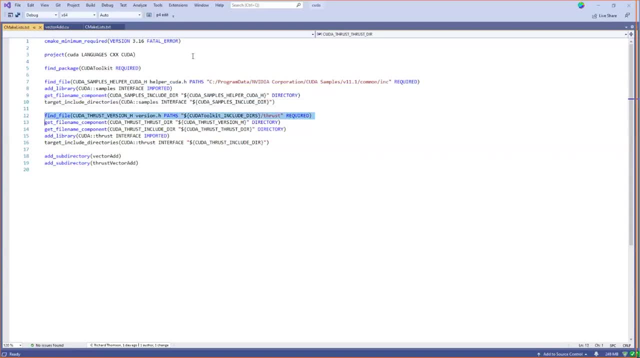 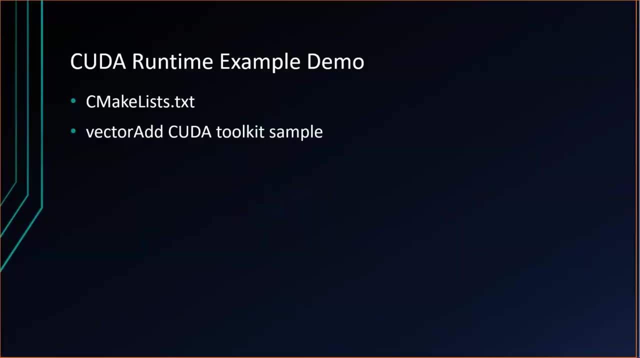 that I just added to my project. That was used in that sample that I copied from the CUDA samples And I set up a CMake convenience for thrust. We'll look at that a little bit later. So the whole reason we're doing this is because we're trying to get concurrency going on to, you know. 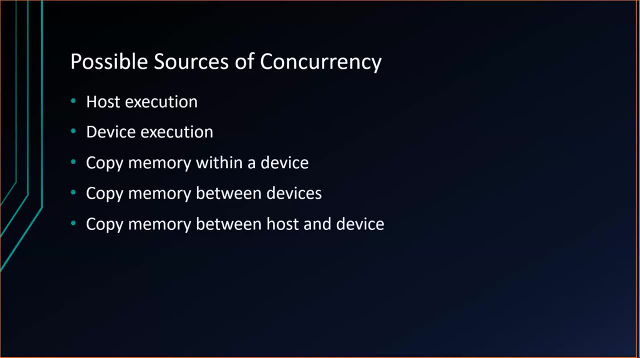 hopefully improve the performance of our application. Or maybe it's just the amount of data we need to process is so large that the more data we can operate on, the faster we can process it, The faster we can get done what we need to do. 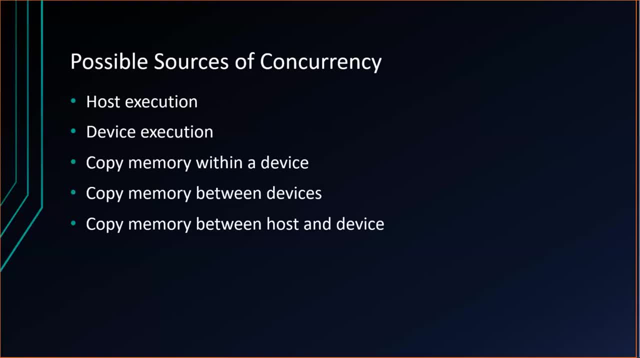 And in any system, if you're trying to get concurrency going, it can be a bit of a problem, because with concurrency always implies possible problems due to sharing of data and coordination of different processes happening concurrently In CPU land. This is, you know, standard threads and things like that. 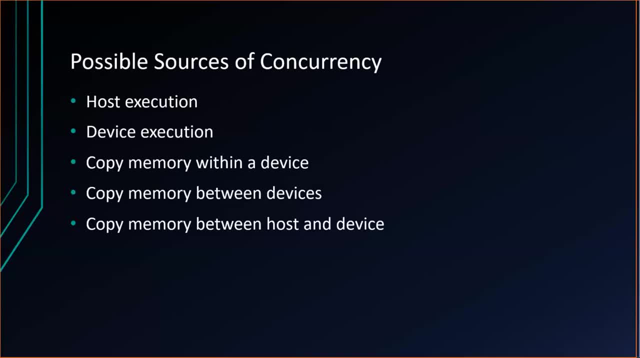 And with a CUDA application there's an extra dimension now of this coprocessor, So we can have multiple threads on the host. That's one form of concurrency we can have going on. We can have code executing on the GPU, So we've got another form of concurrency going on. 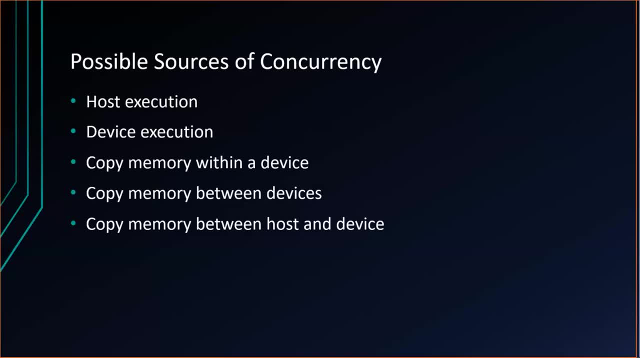 And these GPU cards. they don't just have graphics pipelines and graphics processing units, They also have memory transfer units, So direct memory access units that can transfer data quickly between the device and the host. A question in the chat is that when we looked at this code, let's just go back. 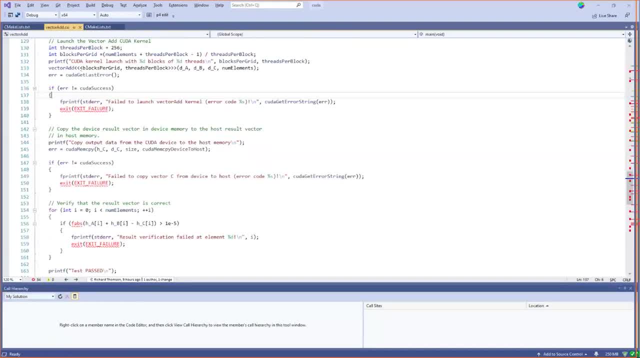 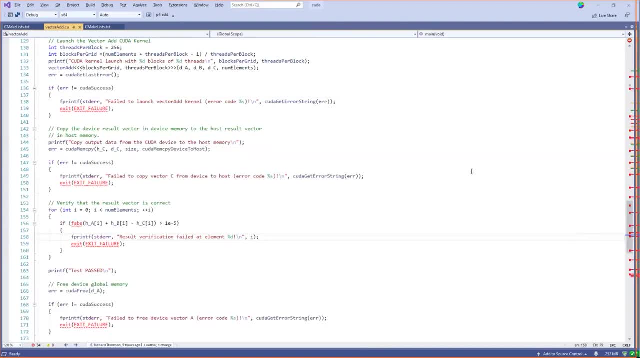 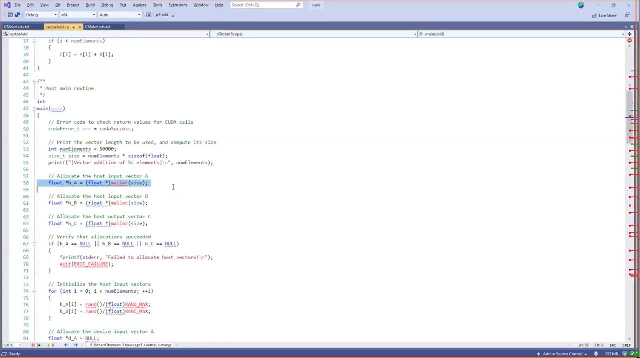 So this code, we were looking here, There we go. And the question is: he sees some mallocs in here and he was right, They were in here when we were allocating host memory. And he says: does CUDA support C++ style new and delete? 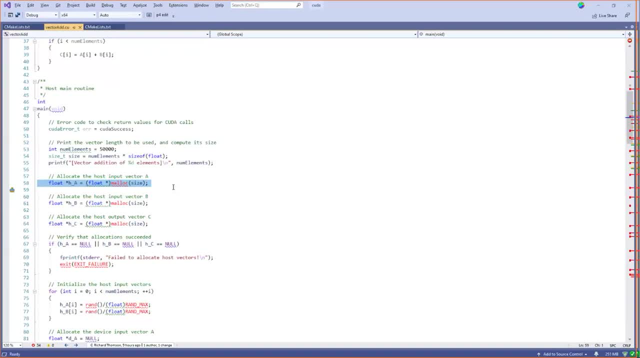 Or maybe it doesn't matter because this would be host code And the answer is in host code. You can use new, delete whatever you want to use In this particular example. this particular example in the CUDA SDK is written in more of a C style. 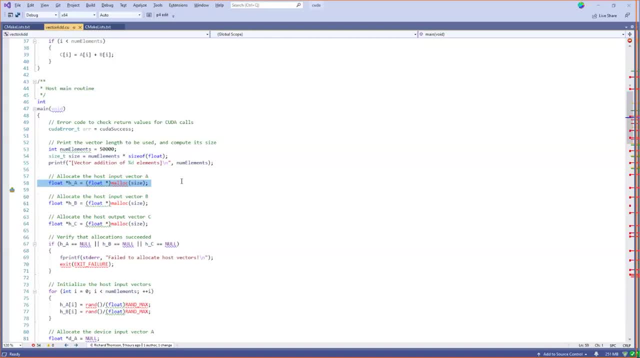 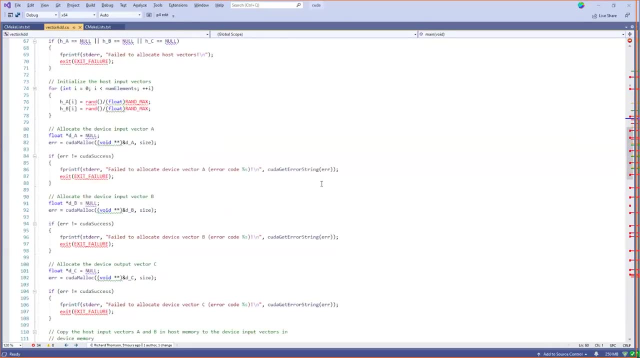 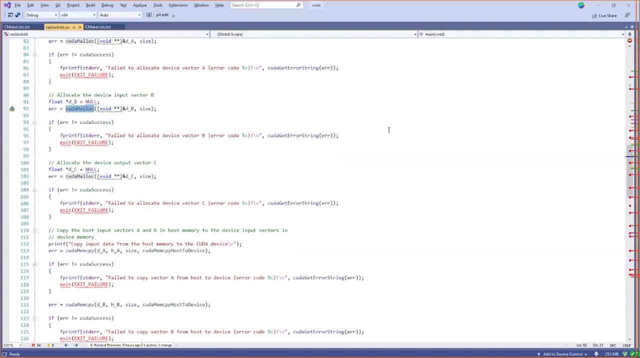 So that's why they're using malloc. But malloc is not necessary here. This is host memory. You can get it any way you want to Down here. when we allocated the device memory with CUDA malloc, that is the only way to get. 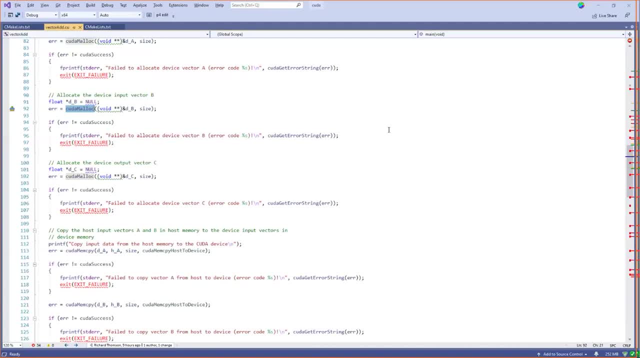 Device memory allocated And device memory is allocated on the host. In terms of- sorry, that's not the right way to say it- Device memory is allocated by the host. It is not on the host, It is on the device. But the function calls that allocate that memory and carve it up are done on the host. 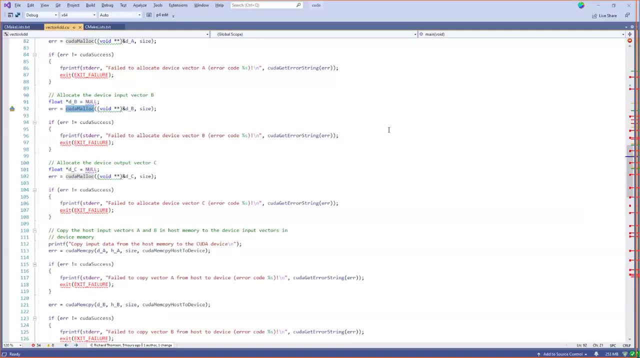 So memory allocation is essentially a GPU Configuration step, not a GPU execution step. I believe that they've got some constrained scenarios where threads running on the GPU could call CUDA malloc, But don't quote me on that, That could be just a mistake on my part. 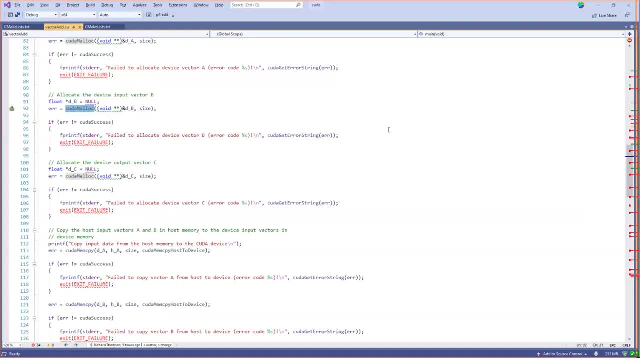 It's very unusual to do that, though, right, Because normally what you're allocating on the GPU is scratchpad work areas, input buffers and output buffers, And for scratchpad buffers, obviously registers are the best. Thread local storage is the next best. 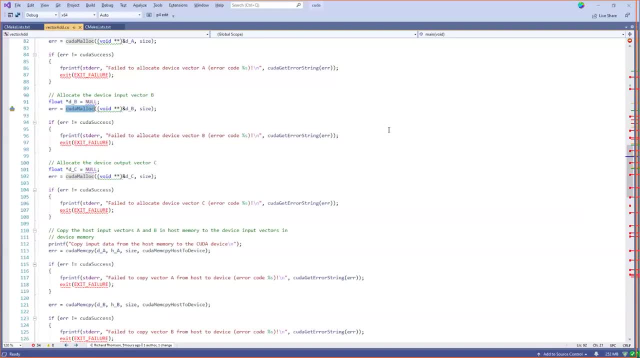 And then shared memory is the next best, And then global memory is what you would be allocating when you run the function calls on the host. So the slowest one is what you get from this CUDA malloc, But basically all the memory allocation is happening by a result of function calls on the host. 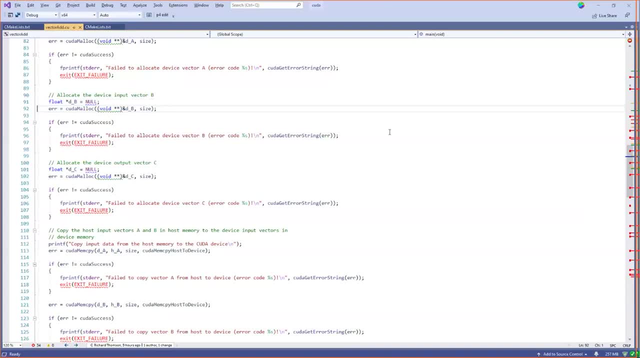 And however you get your host memory is up to you. It could be a shared memory segment, It could be a memory map file, It could be anything. CUDA doesn't care, because it's only used as the source or target of copy operations. 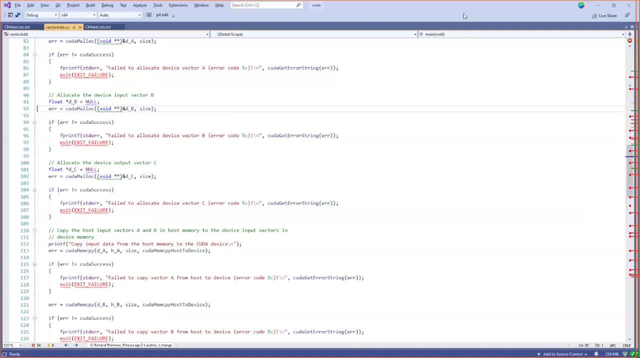 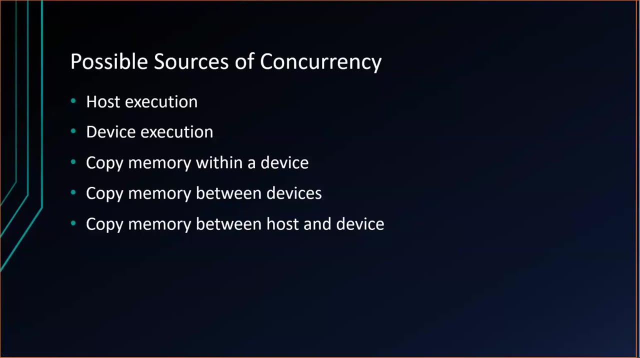 There is advanced usages where you can have a shared address space between the CPU and the host- I'm sorry, between the CPU and the GPU, But we're not going to go Into that depth because this is introduction. So, as I was saying, you've got the execution. that is obviously happening concurrently. 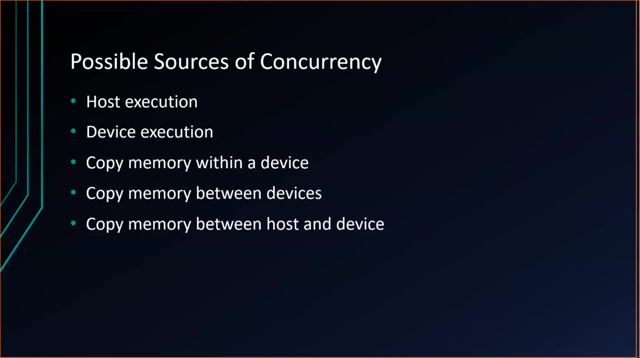 But I can also have these copy operations in flight between CPU. I guess host memory and device memory or device memory and host memory or device to device. You can have copy operations flight in parallel with the execution of kernels in the blocks. So we mentioned 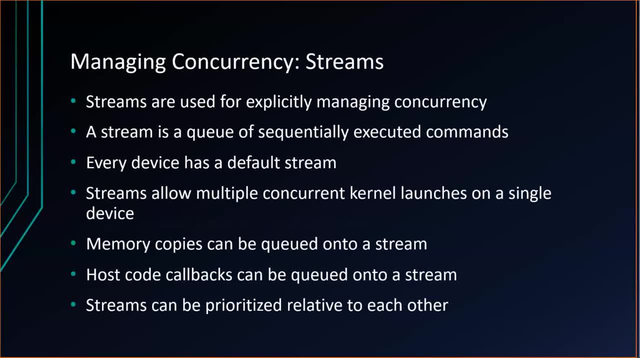 that it's code on the host that is running as doing these memory allocations, it is doing the kernel launches and it's doing these memory copy operations. If you want to get the maximum amount of concurrency, what you really need to do is arrange everything as a bunch of asynchronous operations. 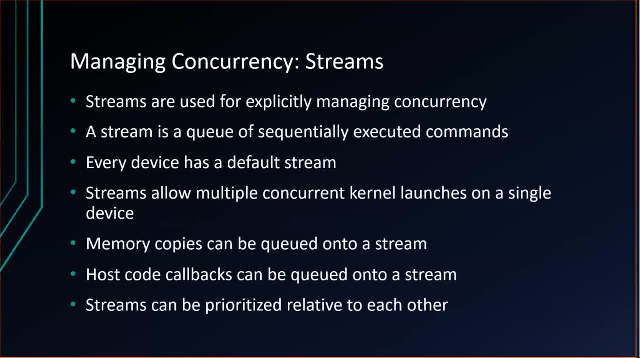 that are happening in a well-defined order, but we don't care about when they complete in terms of the intermediate steps. We just are waiting for the final result to come back to us. However, those intermediate steps may have constraints relative to each other, such that they have to happen in a certain order, even. 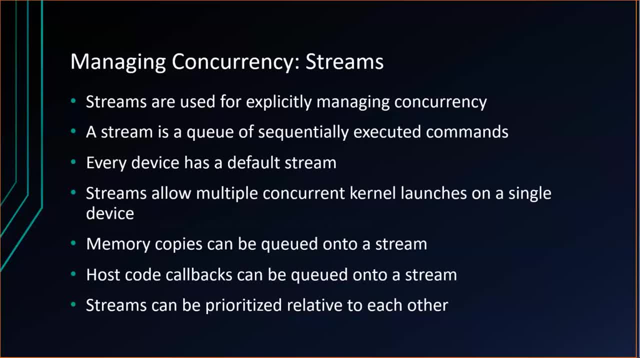 though they've been scheduled concurrently. So, in order to manage that, the CUDA API provides something called a stream, and it is basically just a command FIFO, a command queue, and the commands within the stream are executed in the order that they were submitted to the stream and 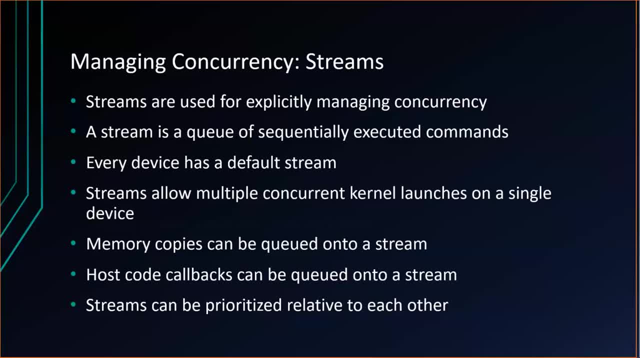 that means that if one of the commands needs something to happen before it can start, it waits Until that condition has been satisfied before that command starts. This is how you can combine kernel launches with memory copies, so that the copies and the kernels could potentially overlap if they're on different streams and as long 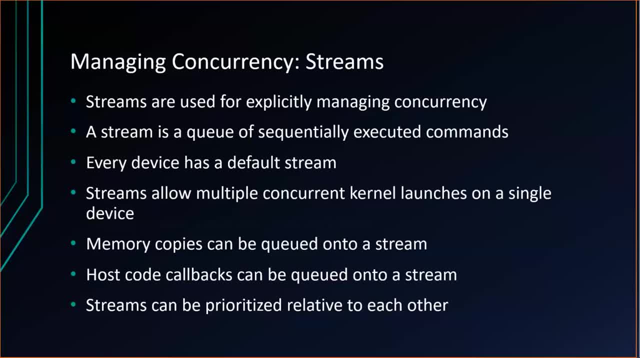 as the kernel doesn't need a copy to complete, they can proceed independent of each other. So this question in the chat said: is there a way to map CUDA results to pixels? And you can do that directly with interop functions that allow CUDA to interoperate. 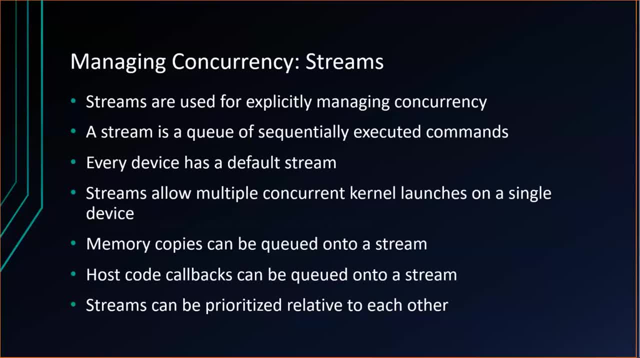 with OpenGL or Direct3D, that you could have. the output of your computation be a pixel surface, a two-dimensional grid of pixels, an image, a texture, what have you in the graphics API So you could just storing into your output. 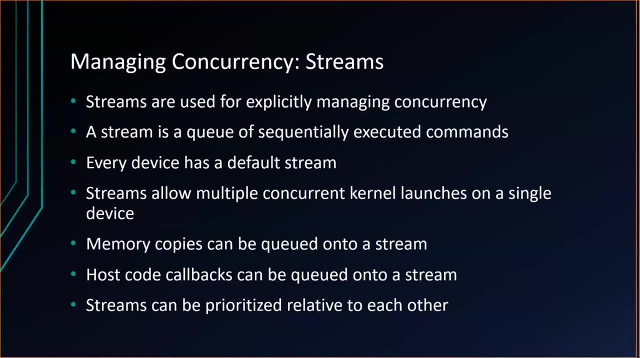 buffer results in modifying this resource that's used in the graphics pipeline. It's really easy to do that. It basically looks from your device code. it looks like you have a pointer to the pixel memory and you are just writing directly into it. 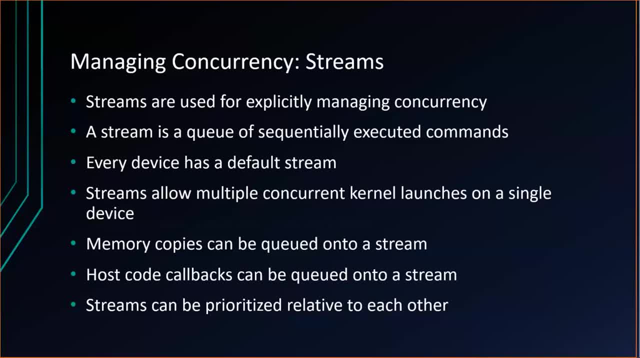 Another question is: is that a typical stack CUDA OpenGL? Let's take a look at this link here. The link's been sanitized and it's not working for me because webex has got the. 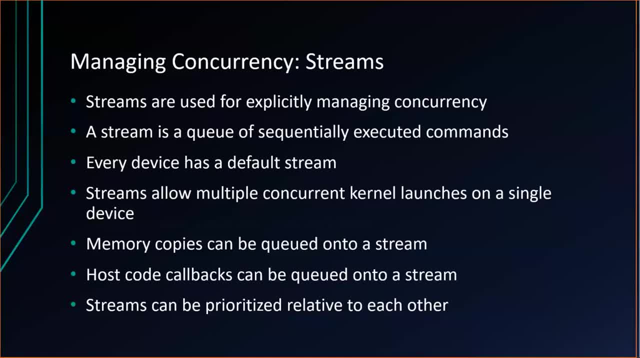 windows all covered up. Okay, so streams are how you can manage the concurrency between different kernels. So within a kernel, you're managing the concurrency by dividing up the problem into a grid of blocks, processing those blocks and combining the block results. 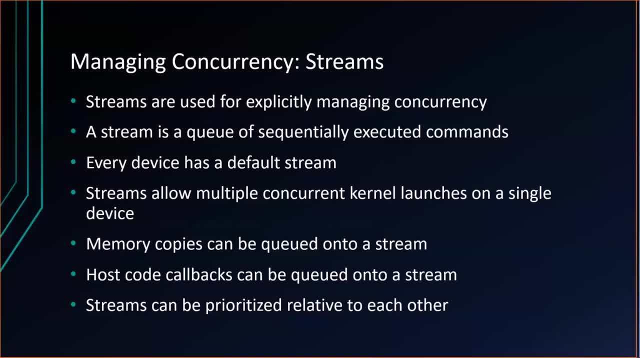 However, it's not always the case that everything you need to do is coming from just one kernel, right? You may have to launch a bunch of different kernels that do different things, depending on the results or depending on your scenario, So you can orchestrate multiple kernels relative to each other, either in a single stream or using multiple streams. 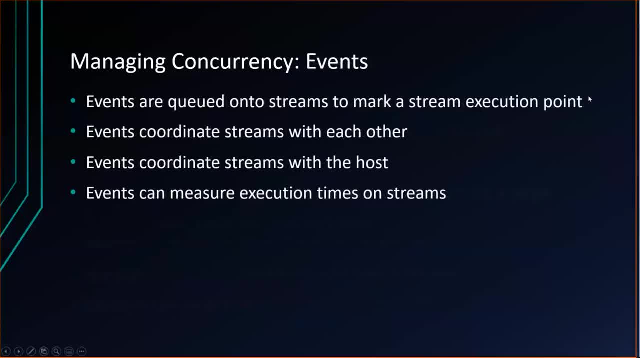 And typically you're going to have, You're going to have additional memory copy events going on to coordinate those events or coordinate those kernels as well. Now for different streams to coordinate with each other, you can use events So you basically can record an event onto a stream and then have another stream wait until that event was recorded. 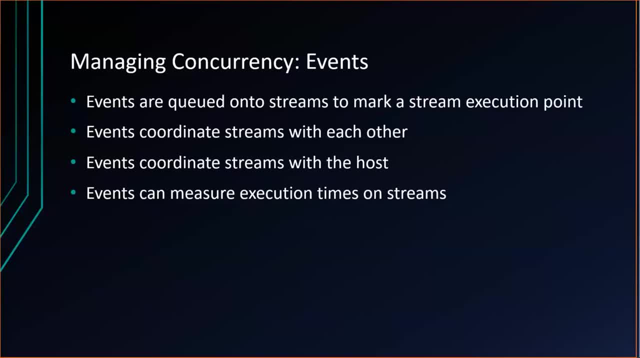 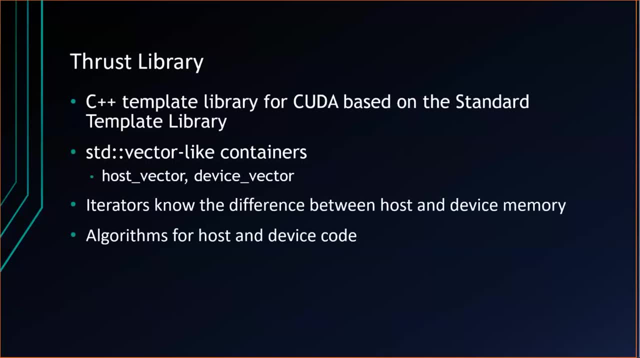 And that allows you to orchestrate the relative ordering of different streams that are operating concurrently in order to solve your whole problem. The Thrust library is a C++ template library that is similar to the standard library in terms of the algorithms and containers portions. 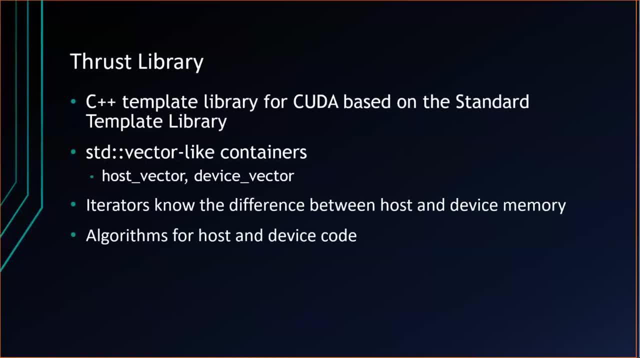 Algorithms, iterators and containers- portion of the standard library And it gives you vector-like containers for data on the host or data on the device And the iterators from these containers understand Which kind of memory they're attached to And they give you algorithms that can operate in host code or they can operate in device code. 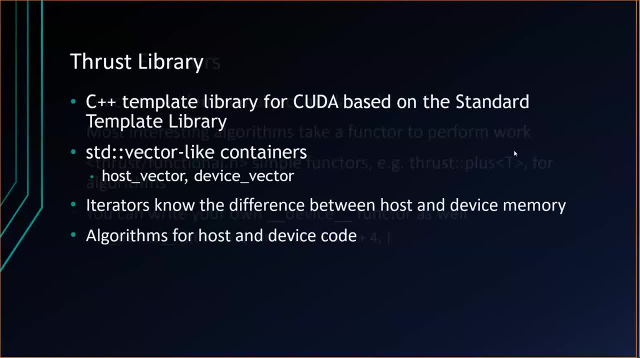 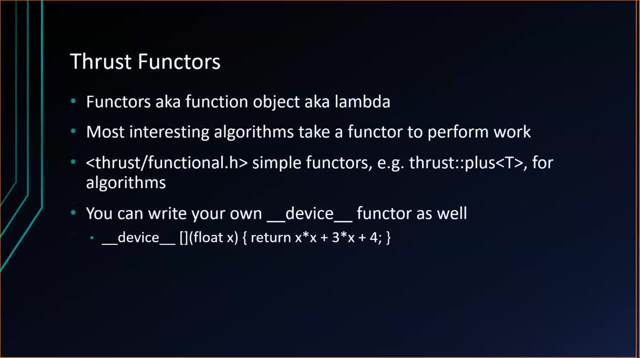 And it works fine either way. Now, generally with an algorithm In order to do something Interesting, Most of the time the interesting part comes from your own computation that you want to do over a sequence or on values within a sequence. 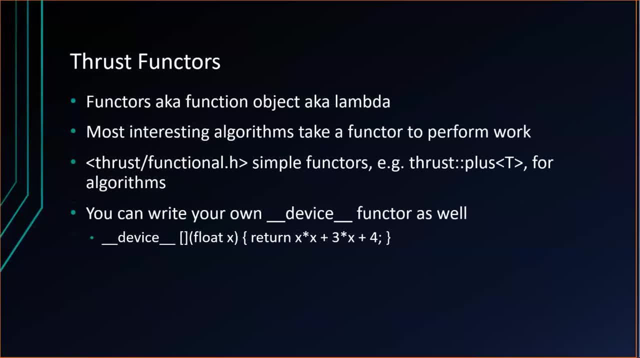 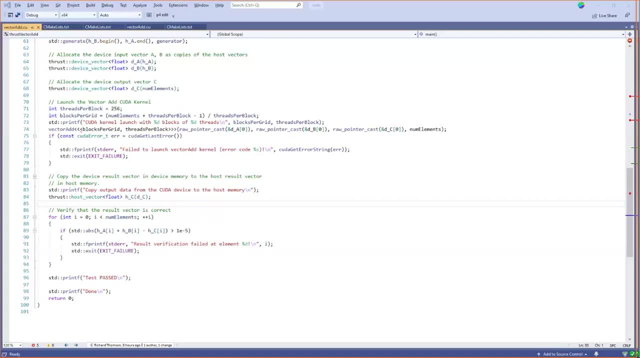 of float in this example, I can just as easily have a device vector of a user-defined data type where the constructor does something non-trivial. What will Thrust do? Thrust will call CUDA malloc to obtain the raw memory. Then it will launch a kernel that invokes my user-defined constructor. 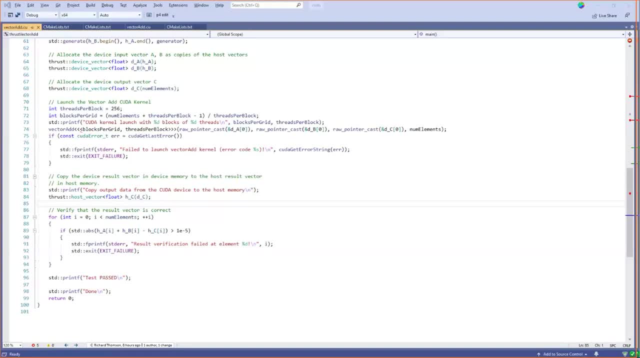 in place on each of the elements necessary to default construct my user-defined type. That's awesome. So it is obtaining the semantics of a std vector, even though the memory that you're manipulating is on the GPU, and in order to run the constructor for your data type on the GPU. 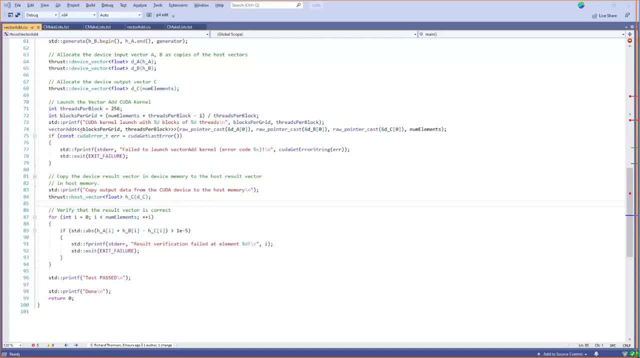 it has to launch a kernel That does the things that std vector does, which is, when you resize a std vector, you didn't give it the value that should be constructed. It default constructs whatever the type is that is on the vector. So Thrust will do that for you, because that's what the 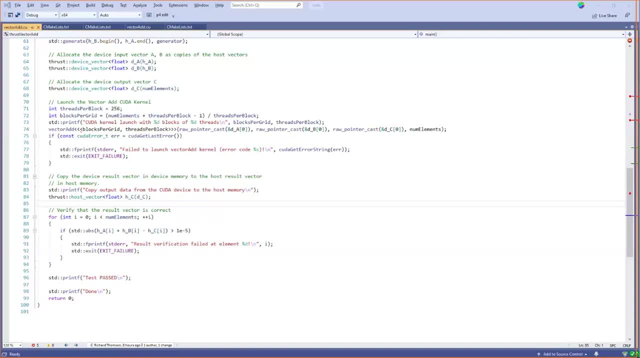 semantics of the vector are. Now, that may be something you don't want to have happen, in which case you can't do that, But it's going to do that for you. In that case, you could just use CUDA malloc, right? 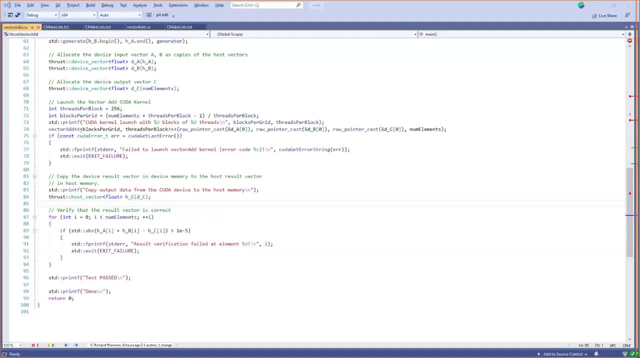 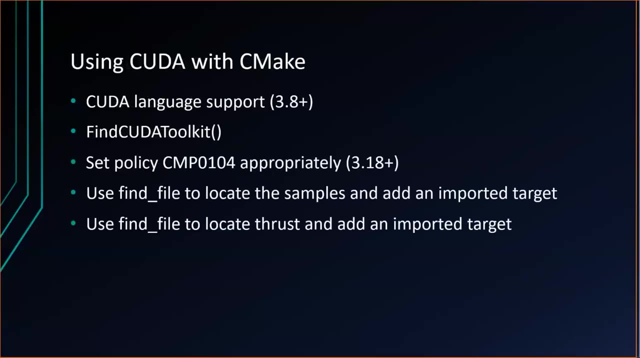 If you don't care if the memory is initialized, you can just use CUDA malloc, because that's what it's going to give you is un-initialized memory. Yeah, that makes sense, Thanks, Okay. so using CUDA from CMake in a modern CMake works really great. 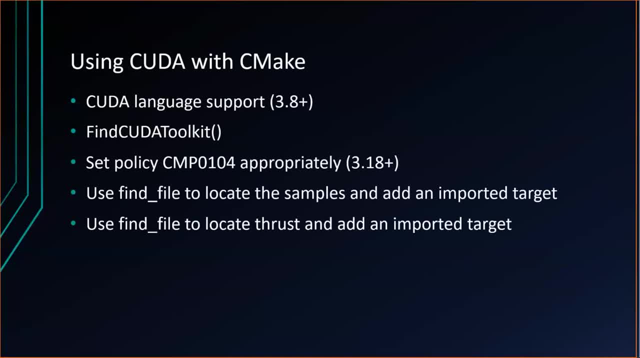 All I had to do was make sure that I had installed the CUDA toolkit after I had installed whatever compiler I wanted to use, because on Windows- and I believe this is Windows, only on Windows- the CUDA toolkit sprinkles in a little CUDA integration into the compiler. 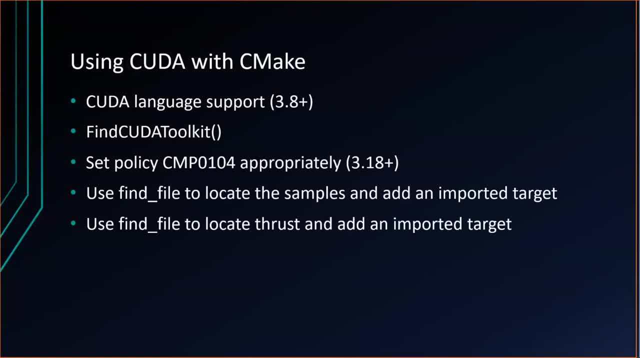 into Visual Studio so that when you run CMake, it can automatically run the compiler, It can automatically locate the MVCC CUDA compiler and it can locate all the binary tools that it needs to run as part of the build process. because, remember, CUDA language support in CMake as long as you have 3.8 or later, which 3.8 is really quite old. 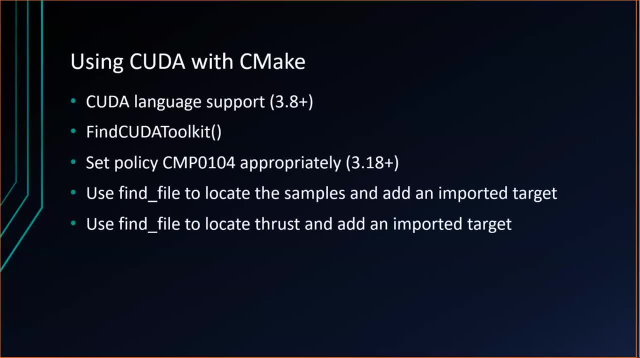 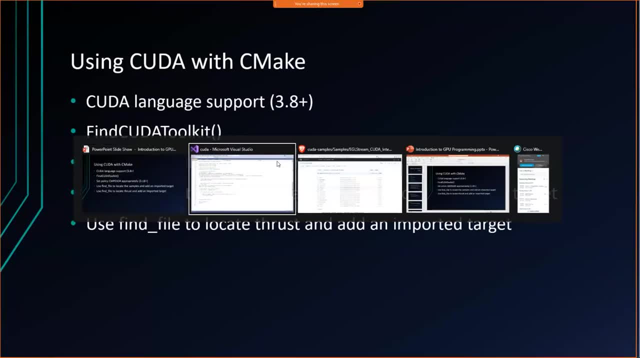 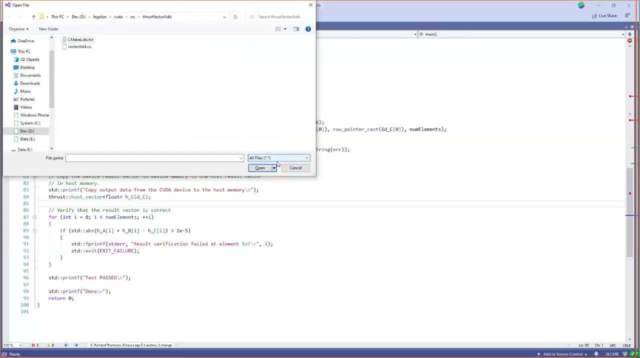 at this point. It's built in there. so when you configure with CMake, we can- in fact we can- take a look. I don't think I have my configure output handy, but in my top-level CMake I mean, I did this. 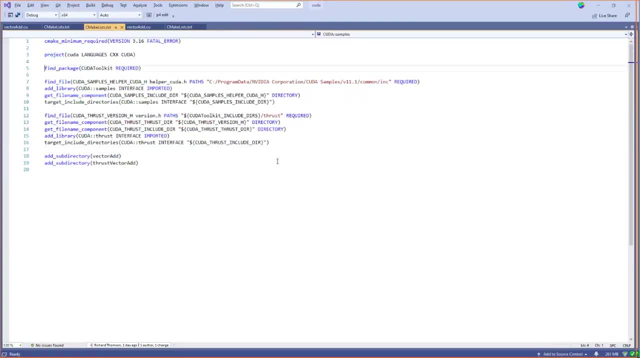 but even saying that I was using CUDA was not necessarily required. and this find package that I did it was just so I could get the CUDA runtime that I link against. but if I was not necessarily needing to do that then well, I guess that's not true. 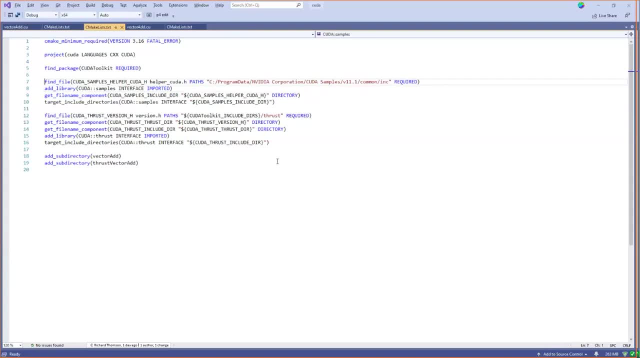 You always need to link against the CUDA runtime if you're using any of the CUDA runtime functions. So that just gave me a nice imported target for the CUDA runtime, but I don't need it to compile a CUDA file. I don't need to find the toolkit in order to compile a CUDA file. 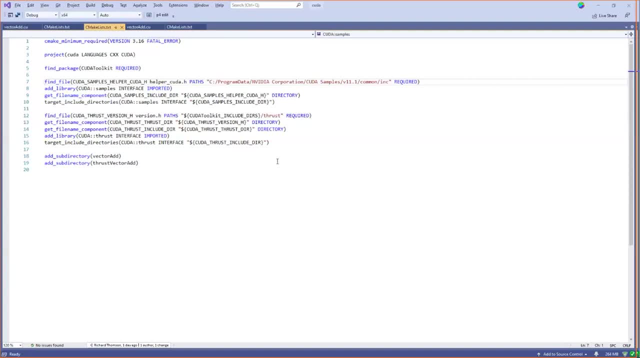 The CMake's CUDA language support took care of that, as long as, like, I installed Visual Studio 2019.. I installed it in particular, So I don't need to find if that's a C++ language support. I don't need to find if that's a C++ language support. 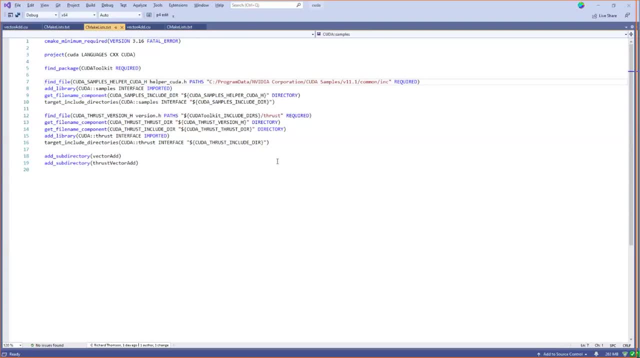 I just don't need to find if that's a C++ language support installed the CUDA toolkit, So at first it didn't work. It said it couldn't find NVCC. but I reinstalled the CUDA toolkit and then it was fixed, So it was really easy. 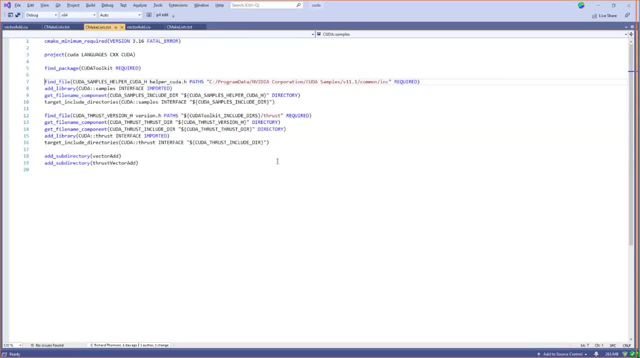 I think linking to CUDA RT shouldn't- sorry. CUDA runtime shouldn't be needed because it will be compiled with NVCC under the hood right. That used to be the case when it couldn't recognize CUDA as official. Well, we can find out. Yeah, All I got to do is go over here. I mean. 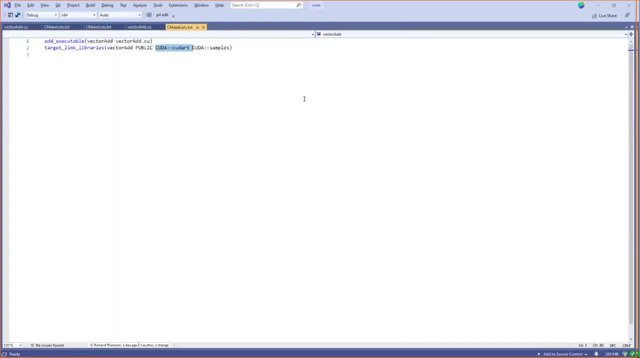 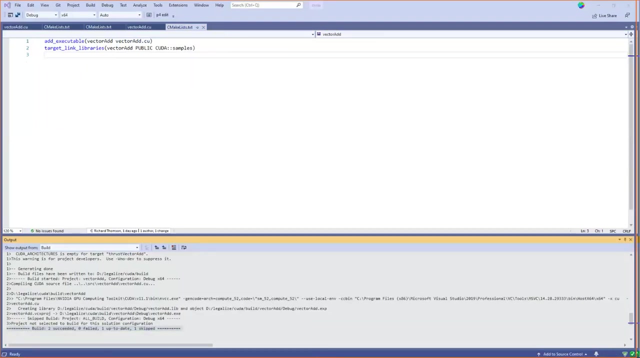 I work on Linux. That might be the only difference. Yay, My Visual Studio keyboard shortcut is bound to something in WebEx. All right, let's just do it this way. I don't know, So it did correctly link. You can't see it until I do this, but it rebuilt, Oops. 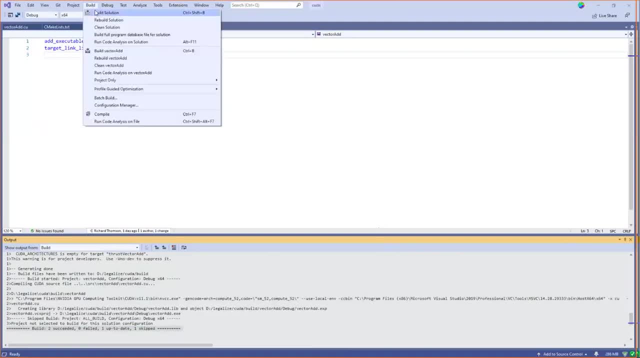 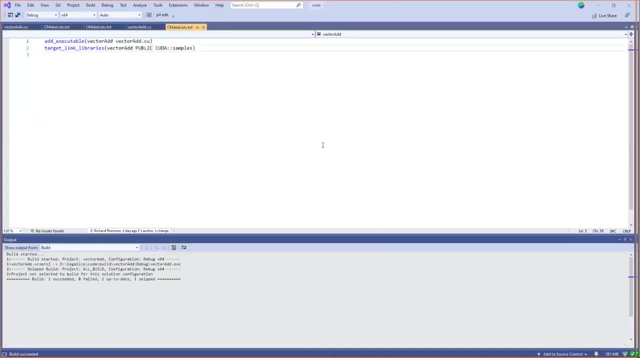 I'm so used to keyboard shortcuts and WebEx isn't liking it, So it rebuilt this sample without linking against CUDA RT. So I think you're right that the MVCC compiler is doing that for you, But suppose I was writing some kind of code. 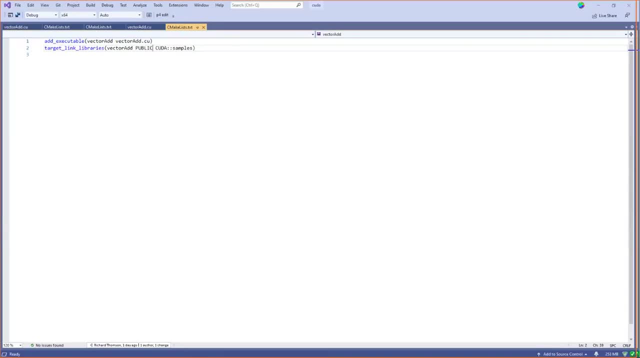 that didn't launch any kernels but still interacted with CUDA, and then it wouldn't be compiled with MVCC because it would just be CPP files. then I would need to link against the CUDA runtime. Yeah, Yeah, So the CUDA runtime is still there. 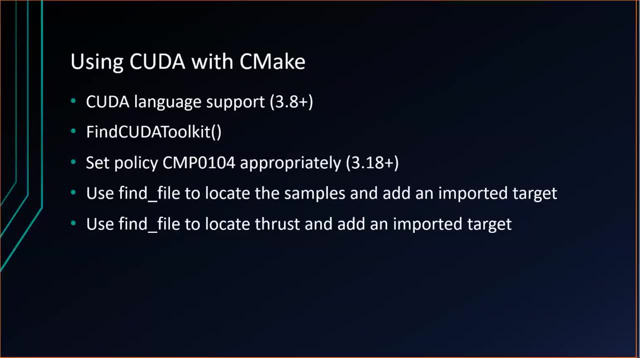 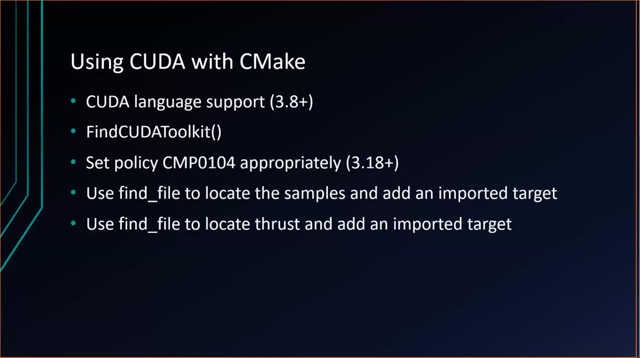 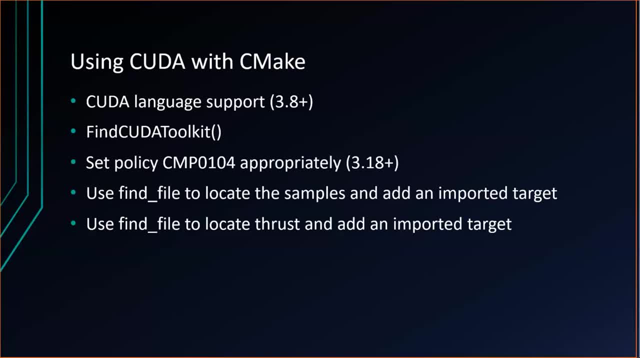 imported targets as a matter of convenience. There is a this policy- CMP 0104, which you might get a warning about when you configure, and it has to do with when we discussed before that your CUDA code, when compiled to the device, it can either can be compiled to a version of PTX, a versionless PTX or a versionless. 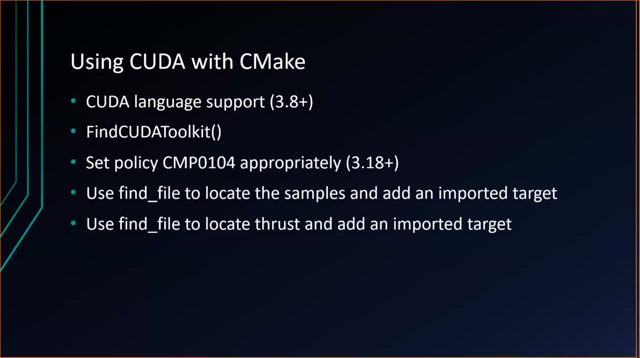 PTX or it can be compiled towards a specific GPU architecture in the form of kubens. They changed the policy saying how the set of default architectures that are targeted by the compiler into a kubin form are specified, And it'll complain to you that you haven't set this variable if you haven't adjusted. 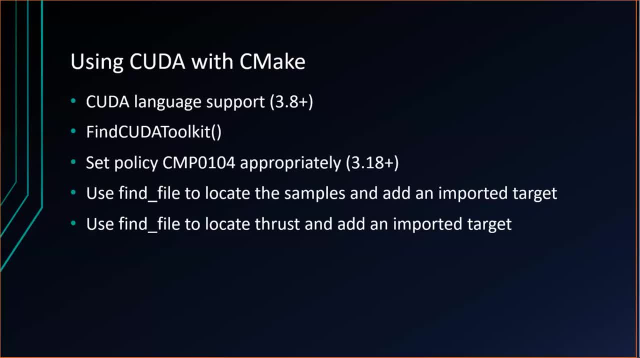 the policy setting. Um, uh, so in the chat there's another question here. It says: is it possible to run CUDA in a hyper VVM? So, um, and another uh comment from a here says: you know, it can work in WSL which. 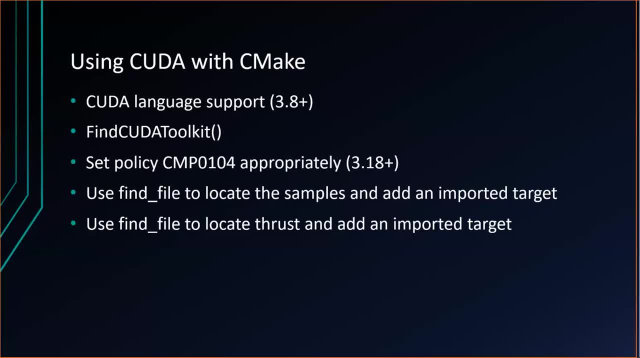 is windows subsystem. Uh, it's the windows Linux subsystem. right, Right, It's the windows subsystem for Linux. That's what it is: WSL. This is basically running real Linux inside windows, With a minimal amount of um VM trampolining in between. 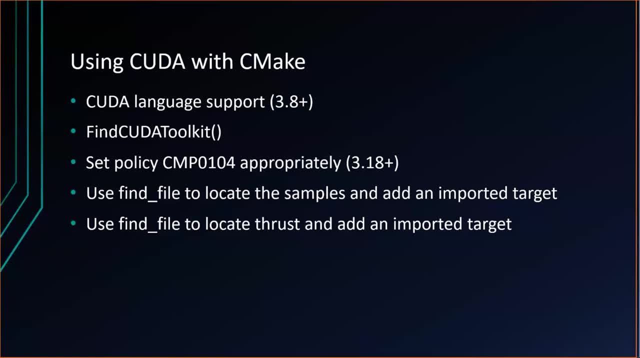 Now they've made some effort in making CUDA visible from WSL And um. that's what me here is commenting on, And the question is: can you run it in other VMs, like in VMware, whatnot? And I believe it's always been possible, but the GPU itself is not virtualized. 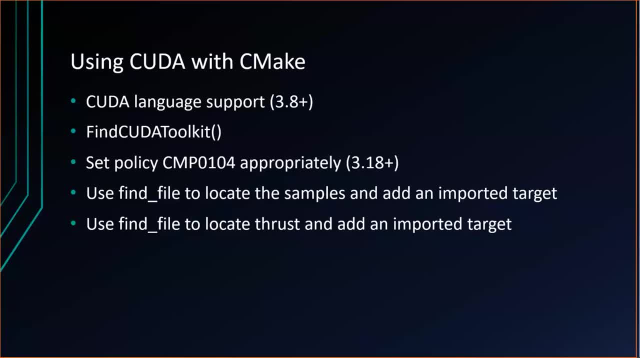 It's not virtualized That. it is what's called PCI pass-through, where a PCI device on the host is made visible as a PCI device in the guest, And that means you can access the GPU uh from the VM, provided you've enabled this. 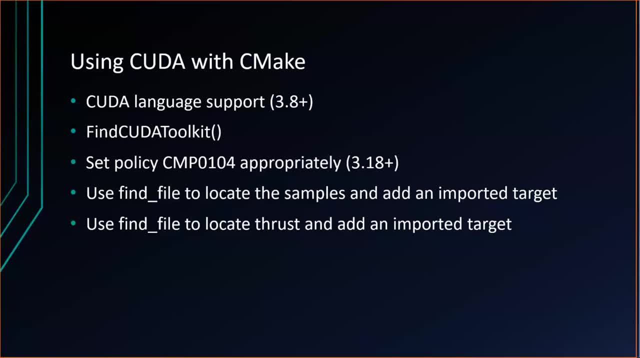 uh, you know PCI bridge functionality, But what it means is um because the access is not virtualized, means the virtual machines can interfere With each other because they're all sharing the same physical GPU. the GPU is not virtualized. 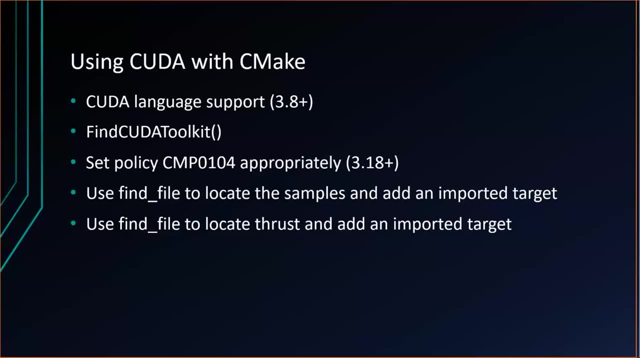 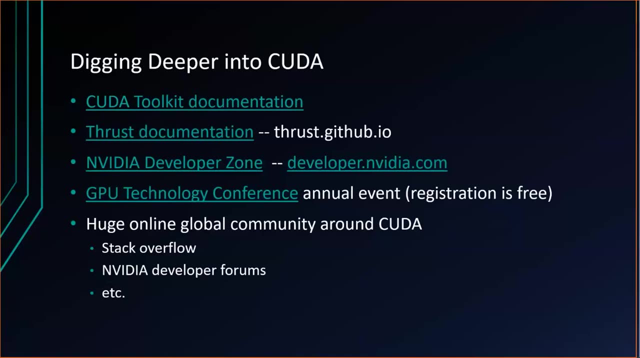 and they can also interfere with the host because, again, the access is not virtualized. Um, so the that policy will be annoying. Just just so you know it's harmless, but like most of those policy warnings are. but if you don't like seeing that output, you can set it appropriately. 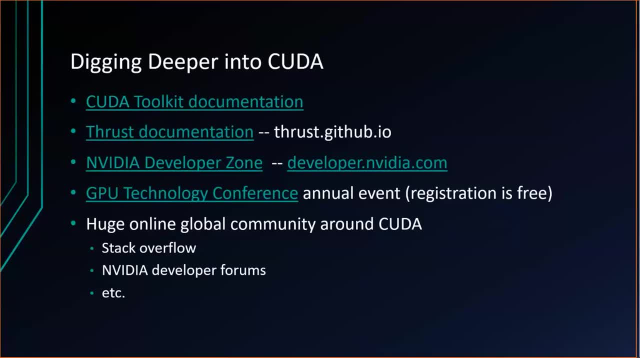 Um, the CUDA toolkit documentation, From which I have lifted examples and figures, is really pretty well written. There's a programming guide, which is where I recommend you start, And from the programming guide you will learn about various uh scenarios and how to uh. 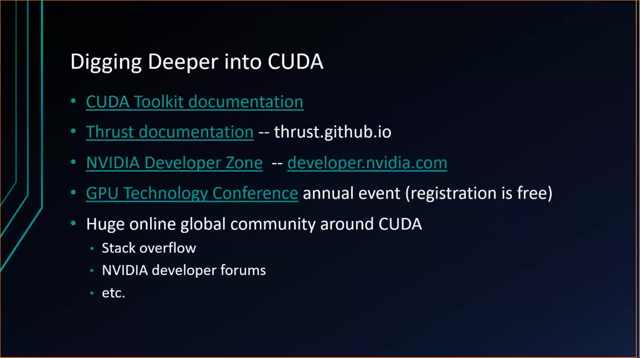 achieve them with CUDA And then from there you can drill into the reference for all the particular functions in order to in their arguments: Um, throw Thrust is also documented in the toolkit, but they have Doxygen-generated documentation up on GitHub so that the Thrust documentation that's in the toolkit gives a general overview of Thrust, kind of like I've done. 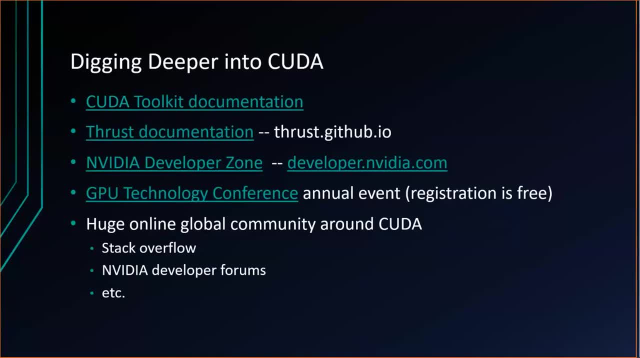 And if you want to drill deeper, then it's off to the Doxygen for you, which you can find on GitHub. Thrust is maintained on GitHub and the version on GitHub may be newer than what's in. whatever, the current CUDA SDK is. 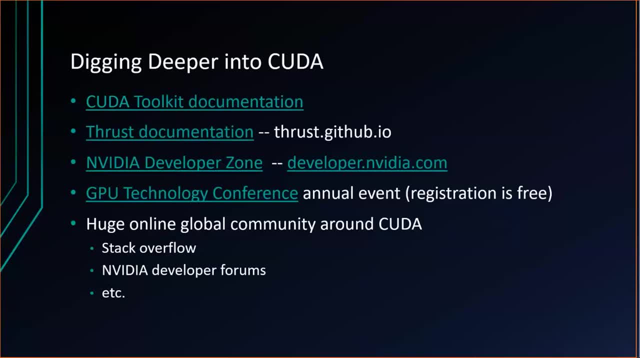 Although the CUDA SDK releases at a pretty good cadence. so as long as you're staying up to date on the CUDA SDK releases, you're not likely to lag very far behind. There's also a huge chunk of- as you might have noticed- Thrust. 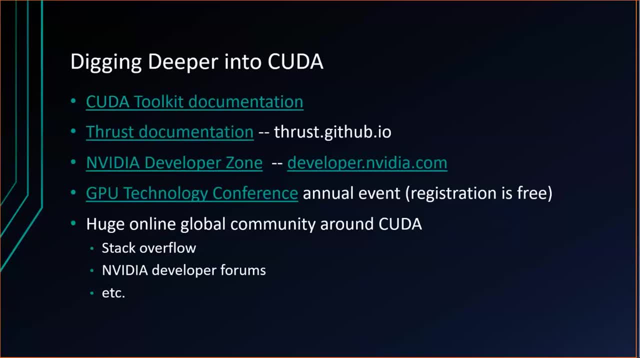 As you might imagine, NVIDIA's website dedicated to developers and it's the NVIDIA Developer Zone. I believe you have to register to join, so, depending on how you feel about giving your email address out, just make a Gmail account or whatever like that, if that's how you prefer to do things. 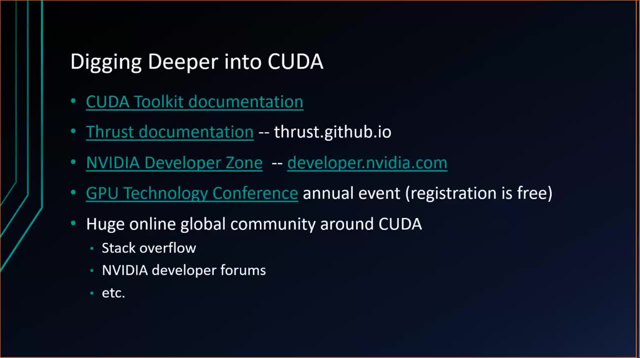 I mean, I've been registered on there and I don't recall getting a lot of- You know- spammy-type messages. but usually the first thing I do after I register is go and turn off all email notifications myself. but you know, whatever works for you guys. 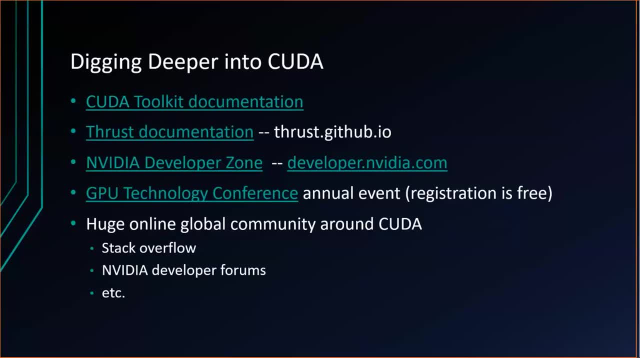 There's also an annual technology conference and I believe all the past presentations are online. You can register for. It's been virtual the past two years, I believe, And it's likely to be virtualized. You can register for Google again, because things are crazy.